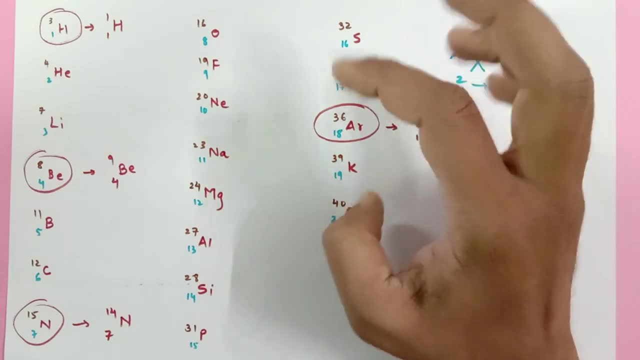 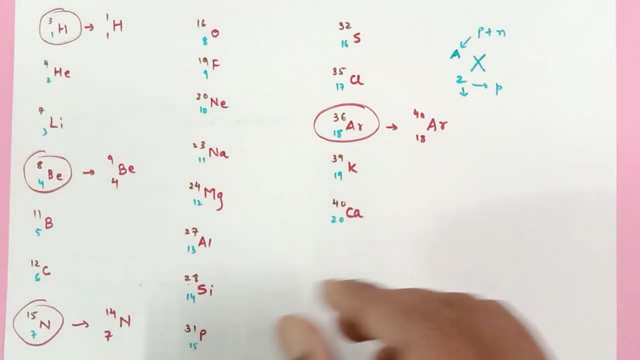 numbers and the atomic numbers. Now I would like to tell you how to identify which of them are metals and which of them are non-metals, noble gases and semi-metals. So for finding the metals, non-metals, or identifying which of them are metals, non-metals, we should 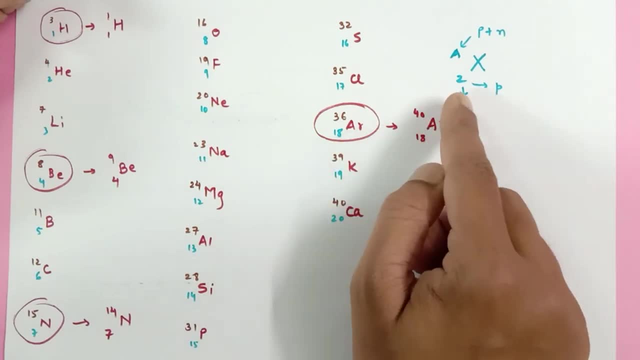 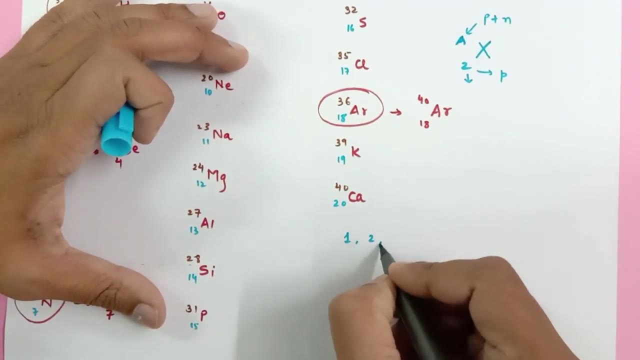 concentrate only on the bottom numbers, which are the atomic numbers. So remember, if you have 1,, 2 and 3 electrons in the outermost shell, or we also say them as valence shell, then they are metals. So for metals in the outermost shell, you should have 1,, 2 or 3. 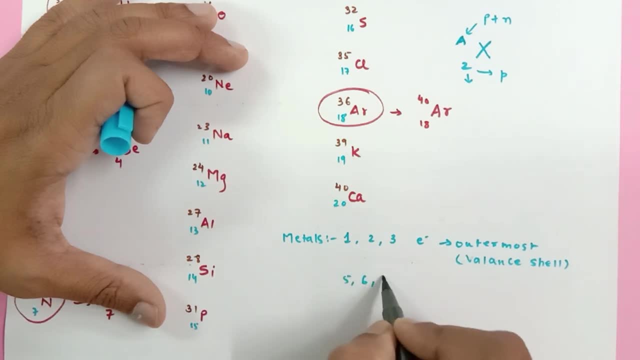 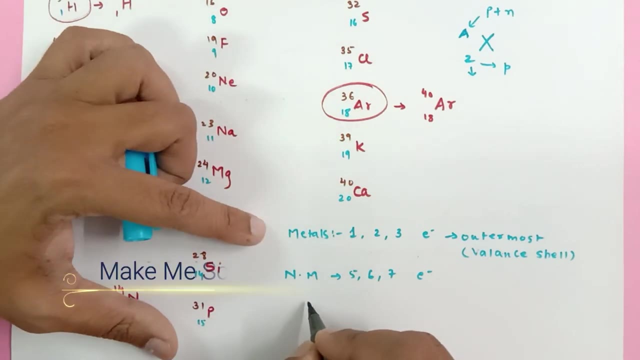 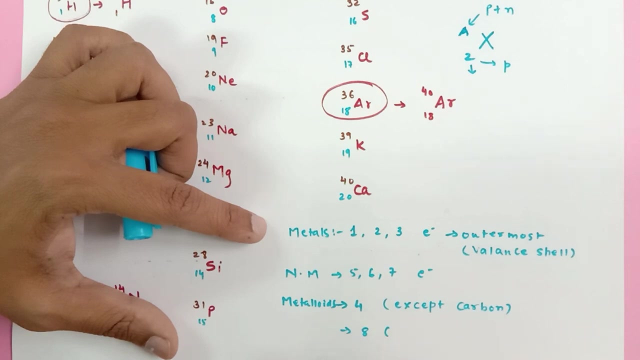 electrons. If you have 5,, 6 and 7 electrons in the outermost shell, they are non-metals. If there are 4 electrons in the outermost shell, then they are metalloids. There are exceptions, as always Like, except carbon, and if you have 8 electrons in the outermost shell, then they are called. 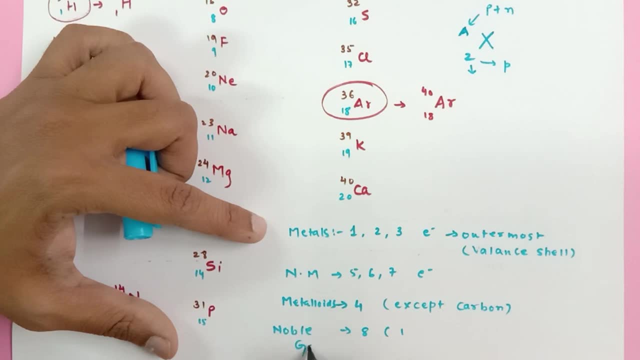 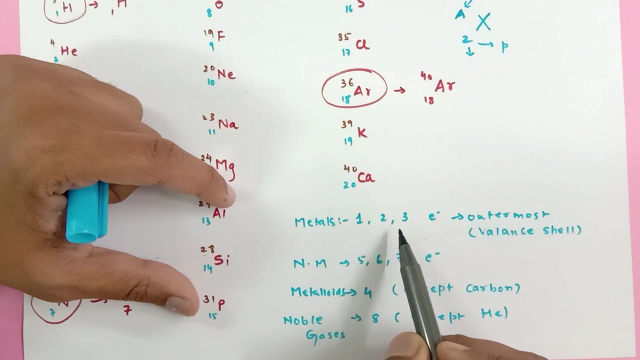 noble gases, Exception again helium, and I will tell you this in quite depth, Right? So in the outermost shell, if there are 1,, 2, 3 electrons, They are metals. 5, 6, 7, non-metals, 4 metalloids, 8 noble gases. 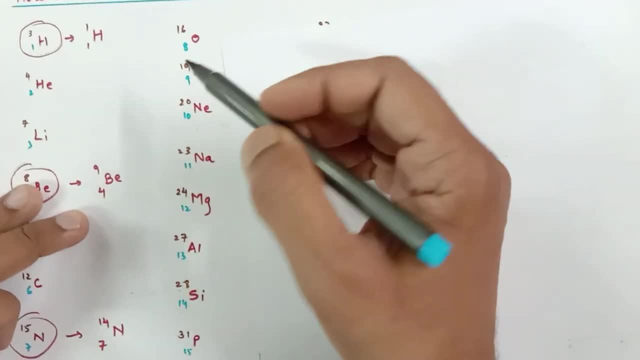 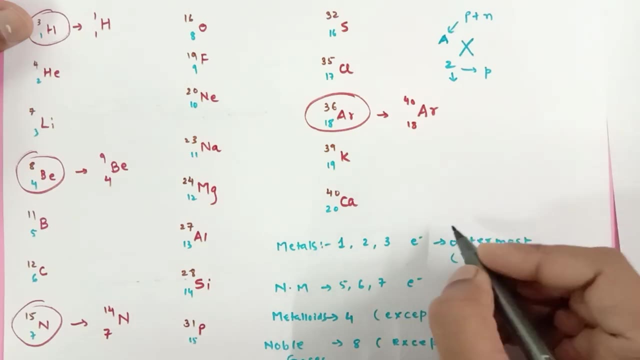 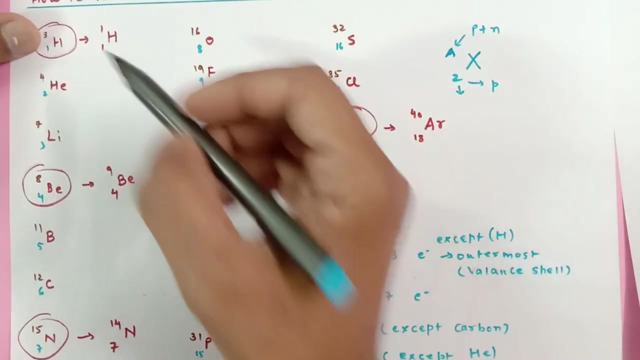 Now let's try to identify them from this part. So in this section, even though yes, I should mention again over here, there is an exception over here except hydrogen Right. So hydrogen electronic configuration is 1.. This is 2. Electronic configuration. 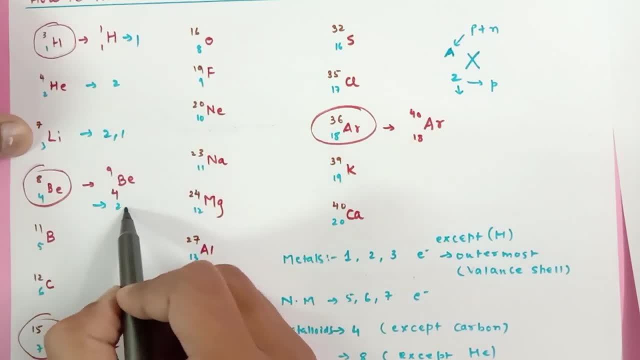 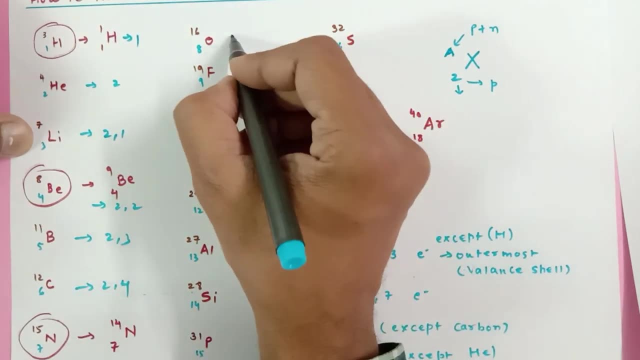 Is 2, 1.. This will be again 2, 2.. This is 2, 3.. 2, 4., 2, 5., 2, 6. 2, 7., 2, 8.. 2, 8,, 1.. 2, 8,, 2., Then 2, 8,, 3. 2, 8,, 4. 2, 8,, 5. Then 2, 8,, 6.. 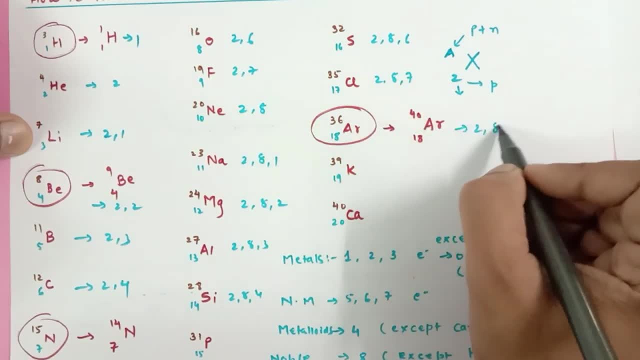 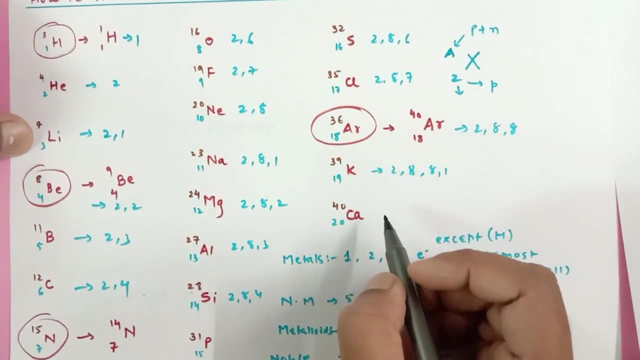 2, 8, 7.. 2, 8, 8.. 2, 8, 8.. 2, 8, 8, 1.. It all together requires a new video for why it is not 2, 8, 9.. 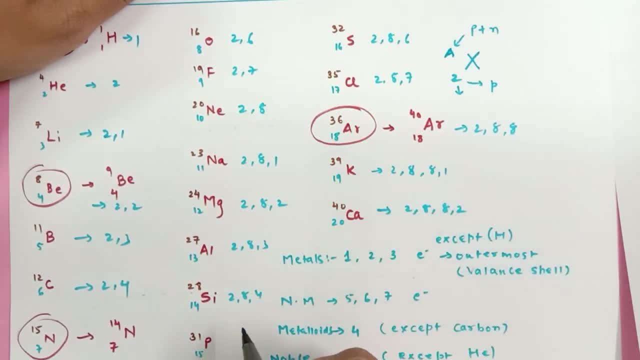 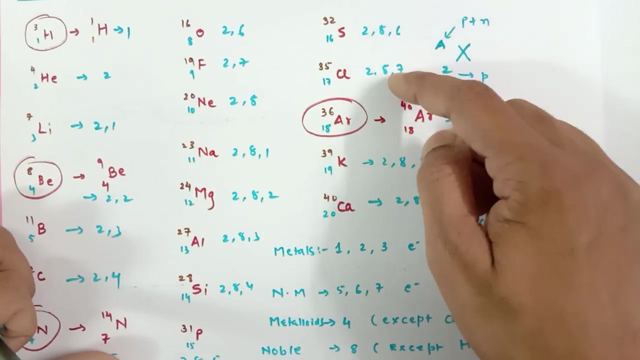 Then it is 2, 8,, 8, 2.. Correct, Okay. Now, as you can see that they have 1, 2 electrons in their outermost shell, So that means these two are metals. As you can check by yourself that they have got 5 and 6 electrons in the outermost shell. 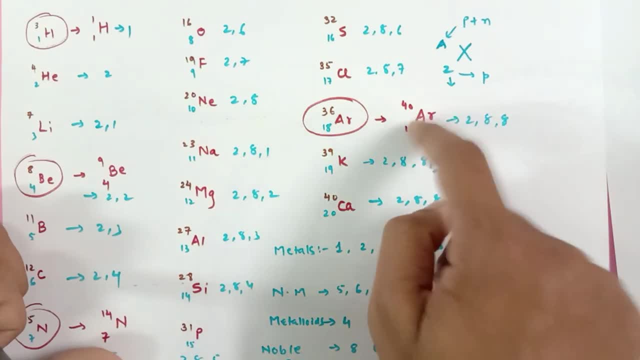 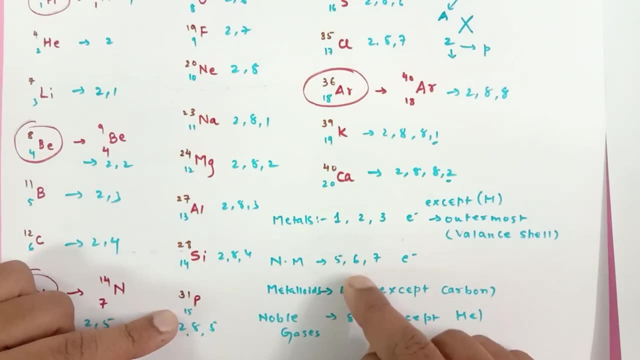 So these two are non-metals. 8 electrons in the outermost shell. So it is a noble gas In the same way. 5, outermost shell in 5. It is a characteristic of non-metal Again. 4, metalloid semi-metal. 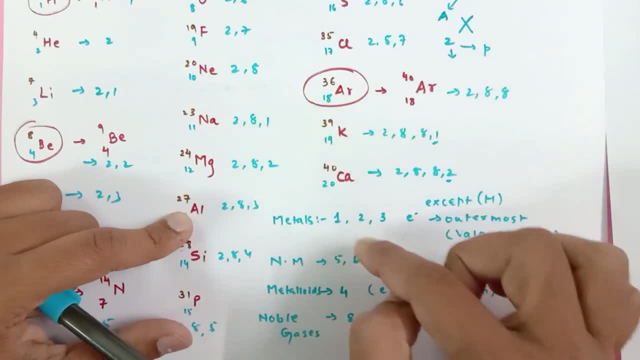 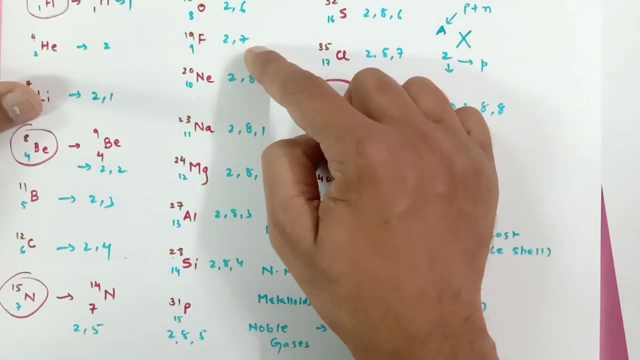 That is half metal, half non-metal. Again 1,, 2, 3.. So these three are metals. This is again noble gas. 6, 7 and 5.. So all these 3.. These 3 are again non-metals. 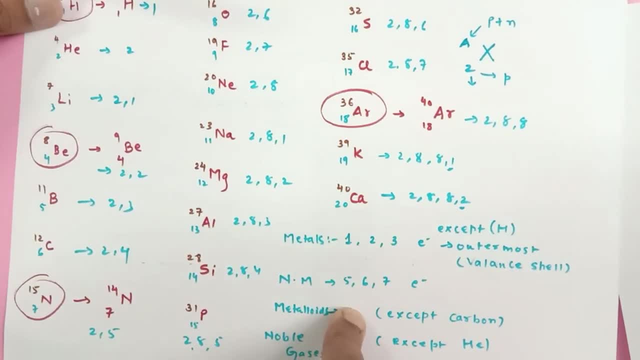 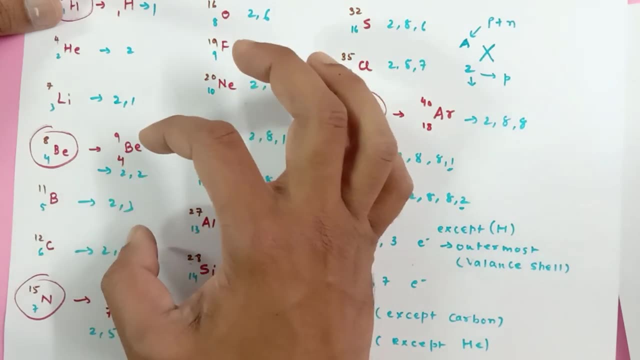 4, even though carbon has got 4 electrons in the outermost shell, it is a metalloid. Now again, sometimes we do consider this in metalloid, but still, for grade 8, it may be fine to say that this is a metal. 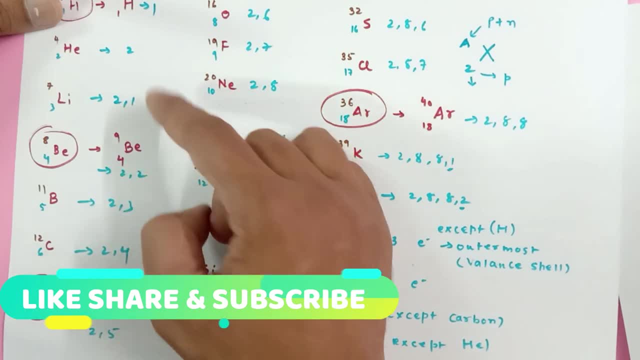 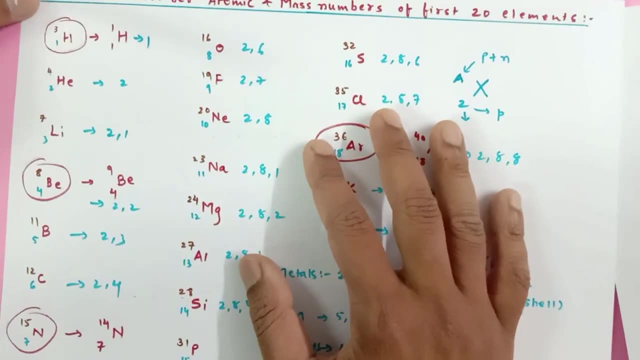 So these- 3, lithium, beryllium and boron- since they have got 1,, 2,, 3 electrons in outermost shell, so can be classified under the metals. This, however, sometimes remains an exception. 2, helium. 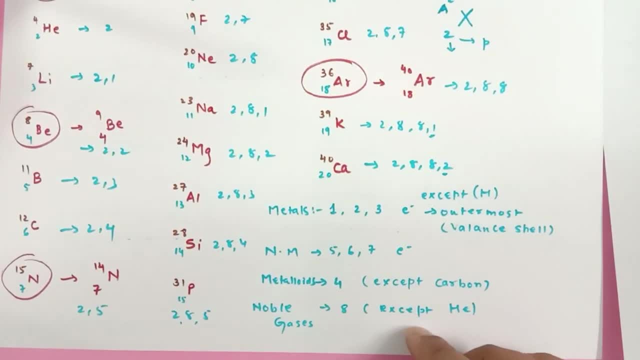 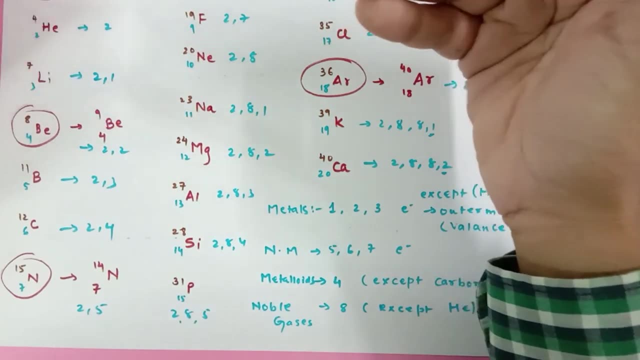 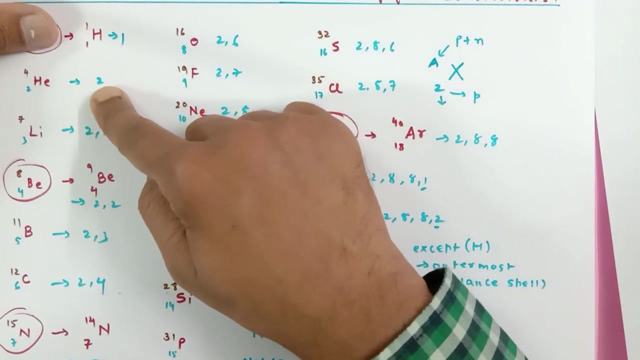 Now why helium is considered in a noble gas. See, noble gas means those elements whose outermost shell is completely filled. Now, in outermost shell you can have 8 electrons maximum. Now, as you can see that this is the first and this is the last shell, 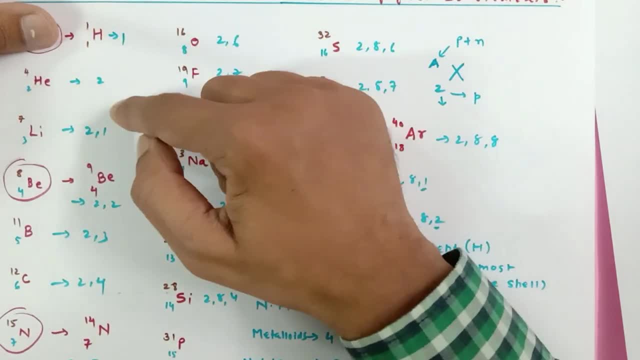 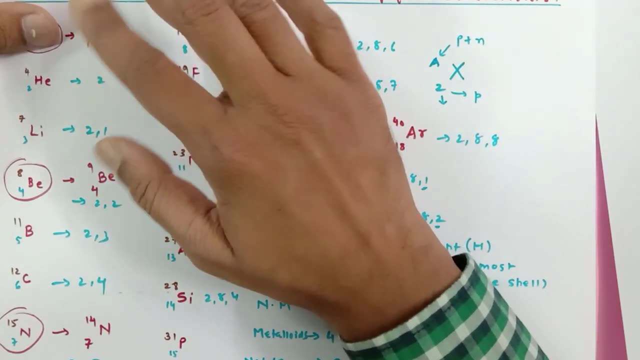 So, helium having only one shell, and in the first shell we know that only 2 electrons can be accommodated. So, anyhow, this helium has one shell, And that is the outermost shell, And that is also completely filled. That's why it is a noble gas. And hydrogen forms covalent bonding. that's why it is classified under a non-metal. Actually, sometimes it behaves like metal. like in acids it behaves as metal, So in acids behaves like metals. Rest in hydrogen molecule in water formation. it is regarded as a non-metal.